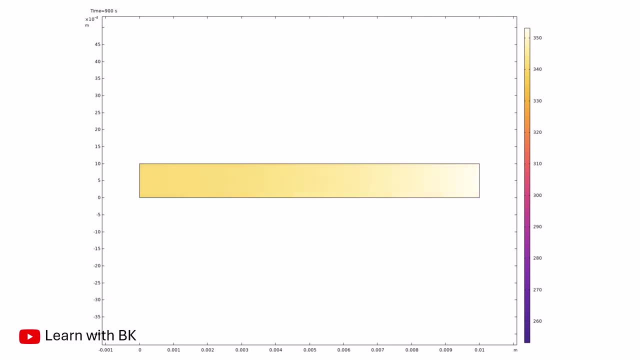 So this is the hypothetical shape of a rectangle, where heat is provided on the right hand side and you can see that ice is being converted into water and we have animated with time. So let us first go through the equation and theory and then we'll move on to the software and learn how to. 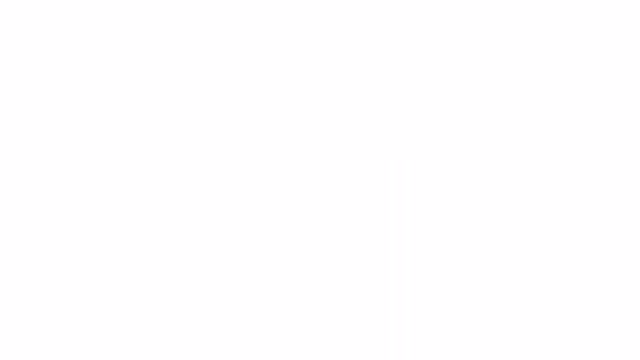 model phase change in the software. So to derive the phase change equation, we begin with the basic heat conduction equation, also known as Fourier's law. So you might know that Q is equal to minus K times delta T. So Q is the heat flux, K is the thermal conductivity and delta T is the temperature. 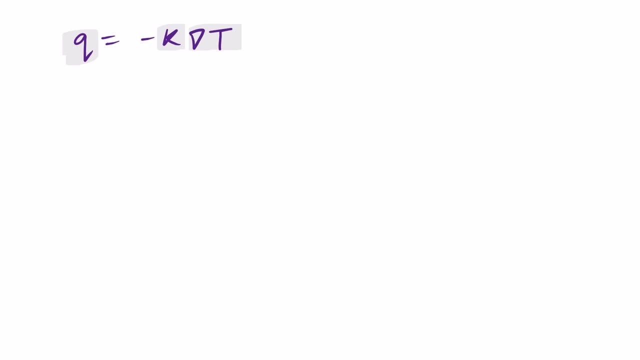 gradient. Now, let's say for a volume element, the rate of change of internal energy due to heat conduction is given by rho, Cp del T by del T, Where capital T is temperature and small t is time, is equal to del K del T. Okay, here rho is the density. 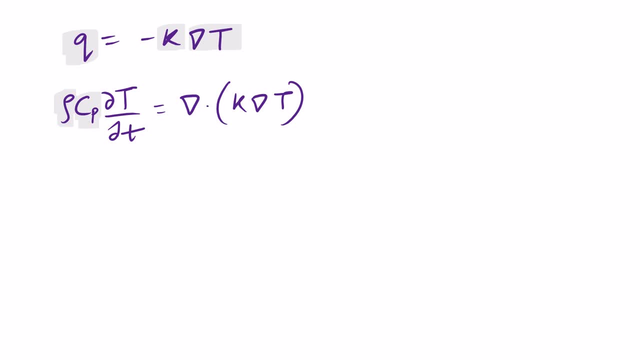 Cp is the specific heat, T is the temperature and small t is the time During a phase change, the material absorbs or releases latent heat without a change in temperature. This is modeled by adding a term representing the rate of energy change due to phase transformation. 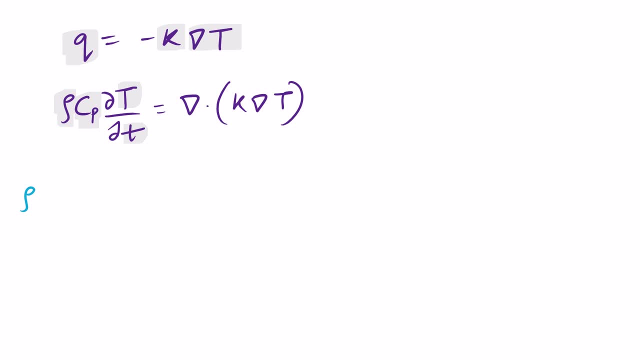 And it is represented as rho L del phi by del T, Where L is the latent heat of phase change and phi represents the phase fraction. Now if we write the complete phase change equation, it looks something like this: So we have: rho Cp del T by dT is equal to del dot K, del T plus Q. 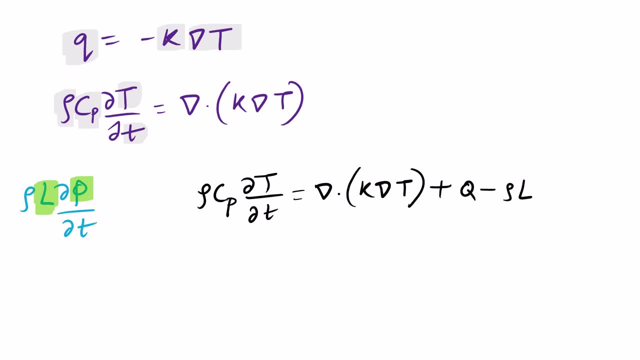 that is the heat minus rho L del phi by del T. Here Q is the internal heat generation per unit. This equation accounts for heat conduction, internal heat generation and energy involved in the phase change. So you can say that this is the complete equation for phase change. So, for example, let's say, an ice cube is 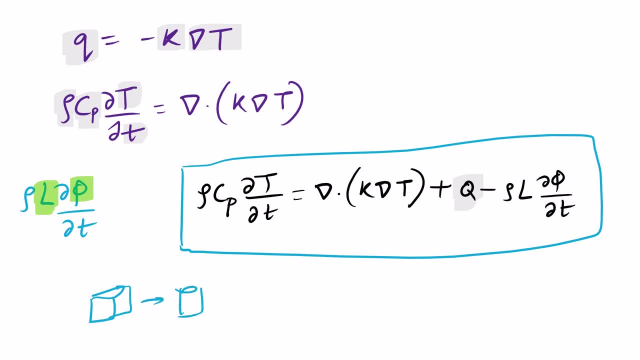 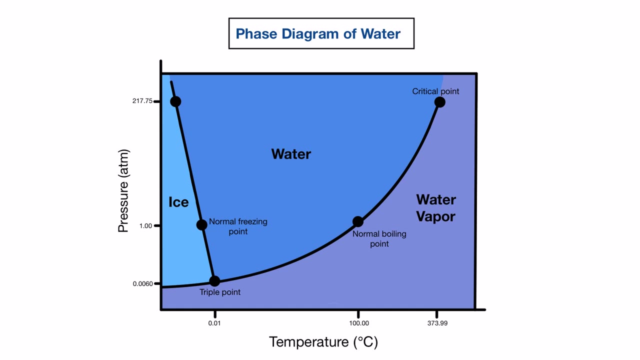 converted into a glass of water, then basically we apply this equation to get the time taken and the different heat exchanges occurring between the two phase change. so before we jump to the software and start modeling the water ice system, let us first understand the phase diagram of water. it is quite 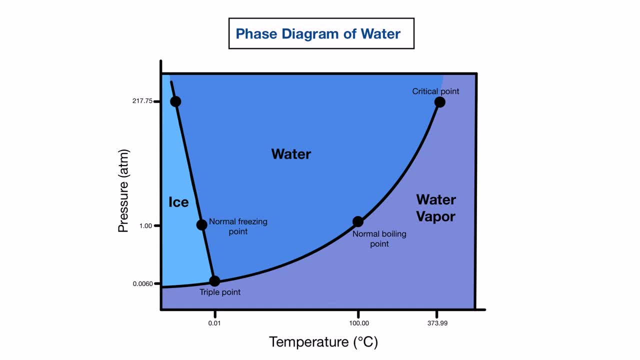 interesting and let us see what we can understand from this. so we have pressure on the one side and temperature on the other. now this is called the triple point of water. this is the most interesting point. that is around zero degree celsius right now as we increase the temperature. 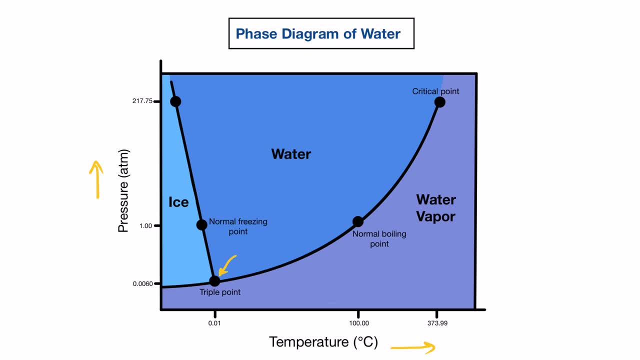 you can see that the water tends to form the water vapor and as you try to cool, it either forms water and as you cool further it goes towards the ice region and at a pressure below a certain limit there is no ice. even if you lower the temperature, it only forms the water vapor. so this is quite a good diagram to understand. 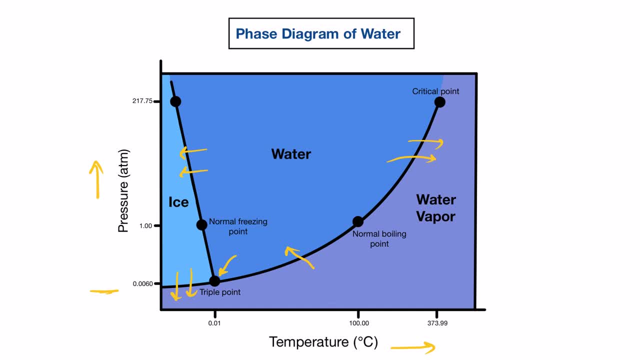 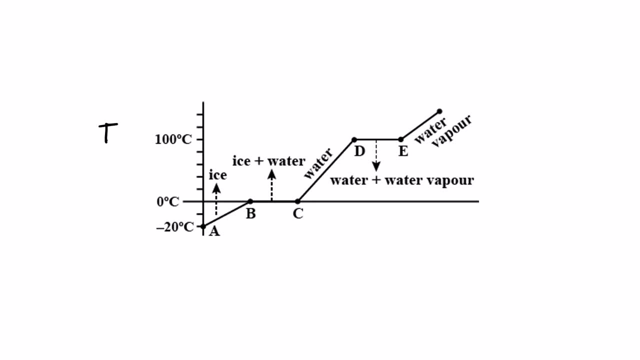 the different phases of water in terms of pressure and temperature. now let us see a different graph where we plot the temperature and here you can say time. so what is happening here? let's say we have a glass of water- basically you can think of it as ice initially- and we are providing some heat and we are actually. 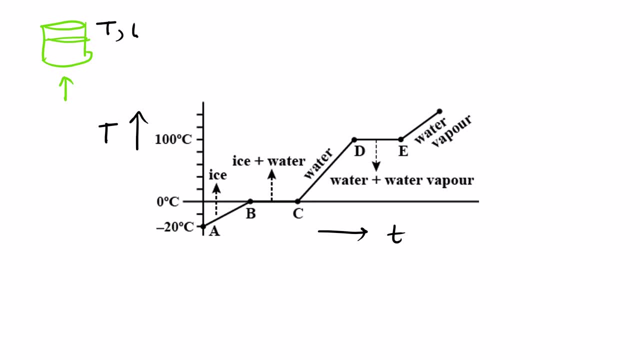 trying to measure the temperature with respect to time. so what is happening here? at first, the ice is at minus 20 degree celsius. then, as we are heating it up, the temperature will rise and at 0 degree celsius, ice will form water. there will be a phase change. since there is a phase change, you can see that the 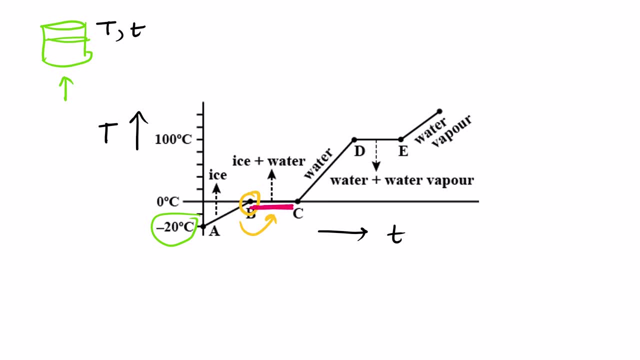 temperature will not rise. all the heat will be absorbed and it will be used in the latent heat of fusion. that will actually convert ice to water and then the temperature of water will rise with temperature again at 100 degree celsius at room temperature and pressure it will again from water to water vapor. so this is again a latent heat. 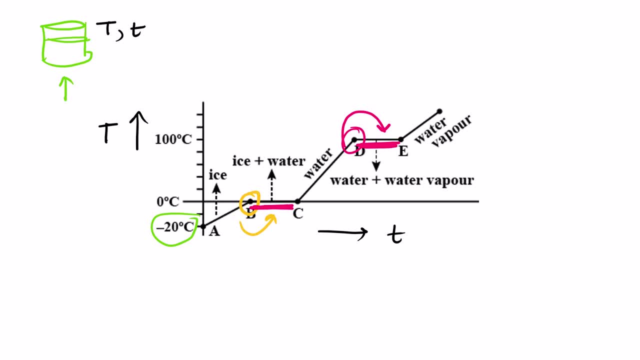 is being used to convert it into vapor, so this is how it works. that is why the graph actually looks something like this. so this flat region are actually due to the latent heat. so now what we will be doing is that we will first take a rectangular block. 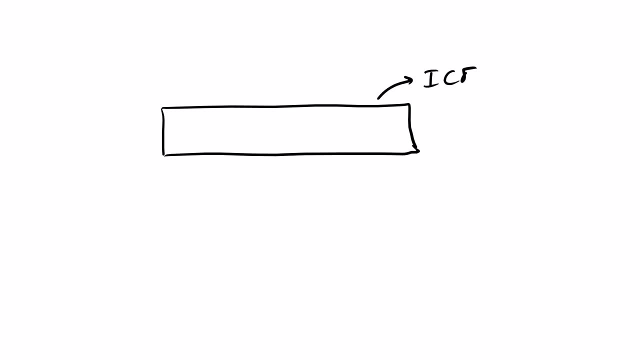 of ice. okay, so this is ice and what we will do. we will provide heat on one side that will basically melts the ice and we will define the density, the specific heat, the latent heat and time and, of course, the dimension of the ice, and we will try to figure. 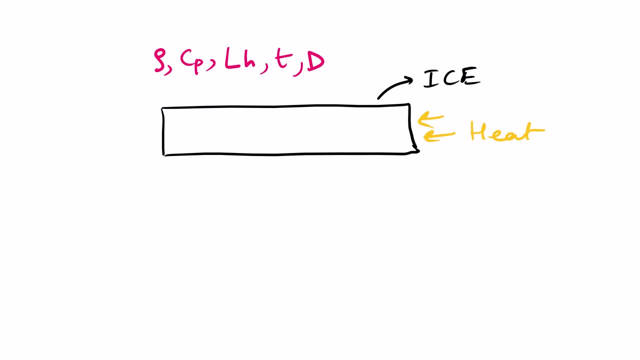 it out with time, how it is melting, what is the temperature profile, heat profile and so on. okay, so this is the main objective of our work and in the meantime, we will also set this as an insulator on the other three side, so that we do not consider the 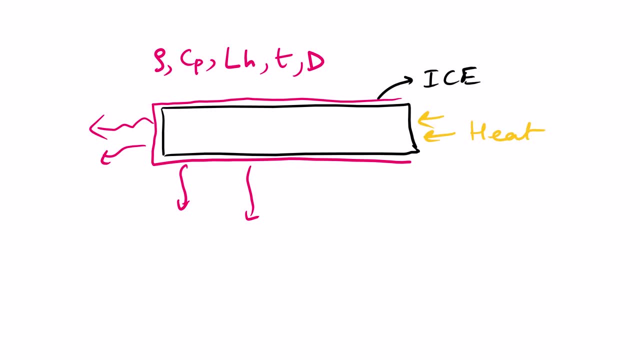 radiation and the other phenomena that are involved in realistic scenarios. so this is how the modeling workflow will begin. so let us jump into console multiphysics and see how we can solve this problem and, of course, if you are interested, uh, to get a python version of this modeling, this can also be. 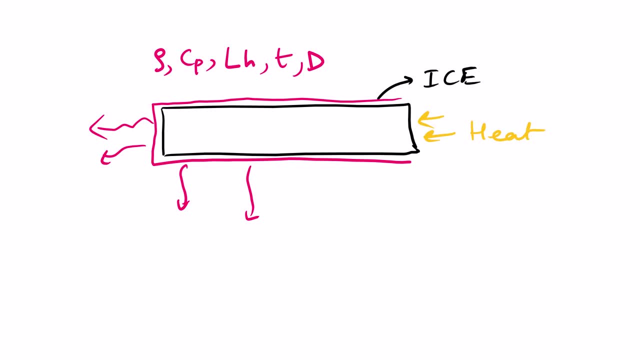 done. uh, do comment in the description if you are interested. then i will create a fully python tutorial of a two dimensional phase change of liquid, totally in python. so let's jump into console multiphysics and see how we can do this modeling workflow. so we are in the console multiphysics window. what we will do first is we'll 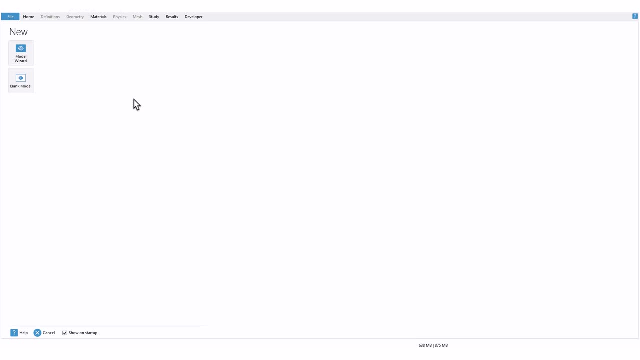 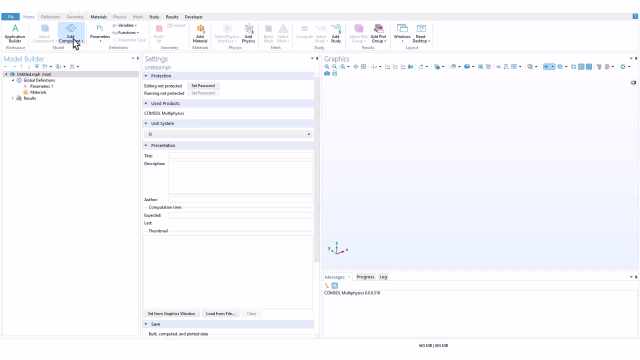 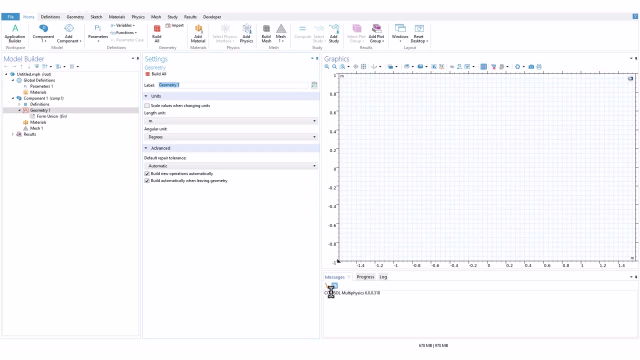 create a blank document and then we'll create a 2d component because we're interested to study our rectangular shaped ice. so we'll go on and click on blank model and we'll just click on add component and then click on 2d component. it might take few seconds. 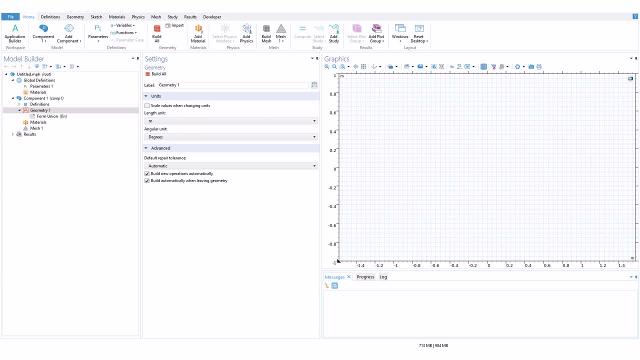 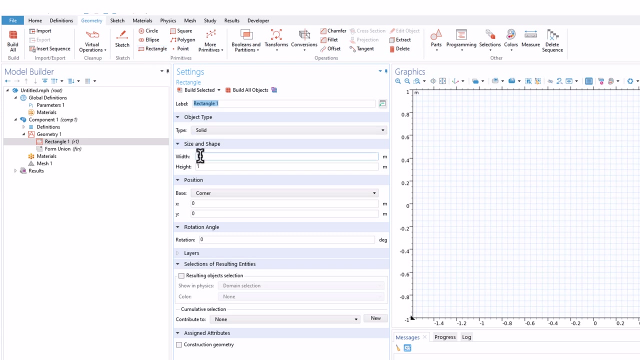 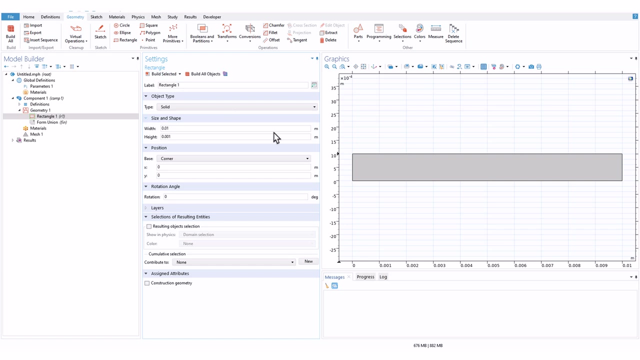 and we'll have the window. so what we'll do, we'll first draw a rectangle and then we'll add different settings. so we'll go on to geometry and then we'll click on rectangle. in the width component we will, I will just write 0.01 and height 0.001 and I'll click on build selected. so you 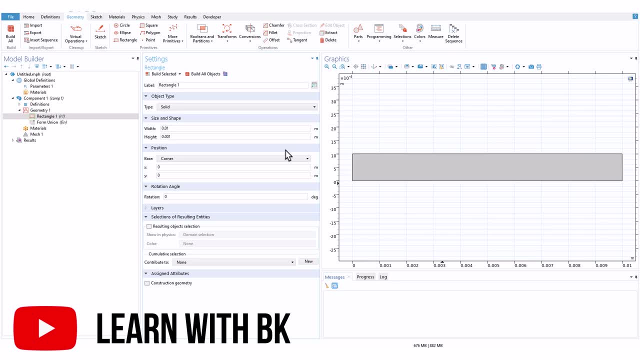 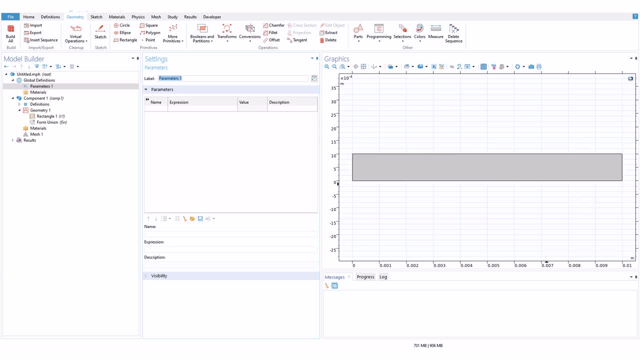 can see that we have the block ready. now we'll go on to the parameter and just add different values that will be needed in our workflow. at first we'll add the transition temperature, so we'll write T trans and this is 0. okay, so you are. 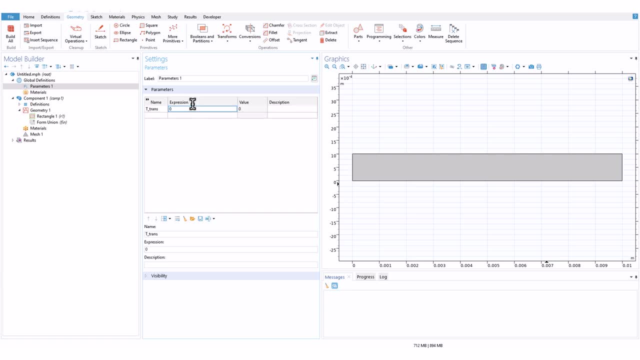 writing in Celsius. so what we can do, we can just write as DGC: okay, that means that this is in degree Celsius and the value will be converted into Kelvin, and now we will add the lower temperature, so T 0, and this is minus 10 degree. 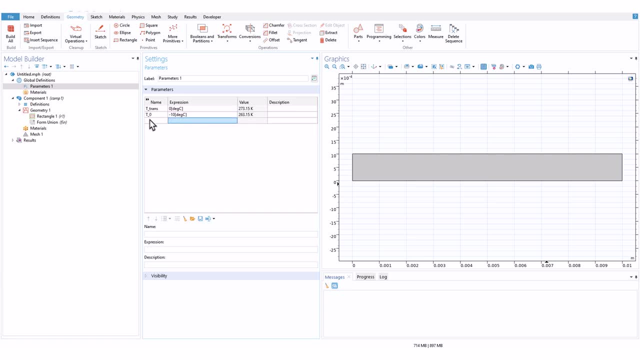 okay, and let us set the temperature of the hottest side, basically the region where we are actually providing the heat. so let this be 85 degree Celsius. so all this temperature are done all together. now let us write the density of ice and water that will be need needed. so density of ice is nine one eight, and of 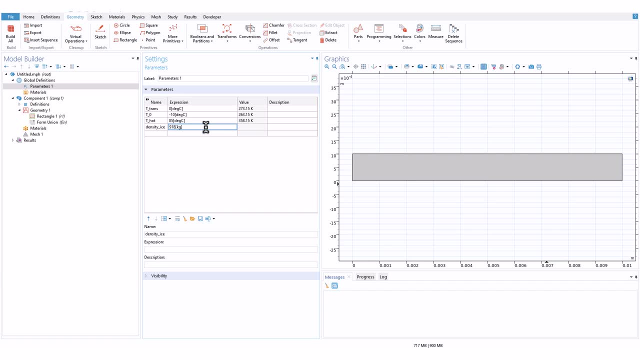 course we should try the unit. so this is kg per meter cube. I'll just copy this. and density of water is 997, or let us take thousand for simplicity. of course you can change the value in your modeling workflow. that doesn't matter, and then we'll also write the ratio of water. 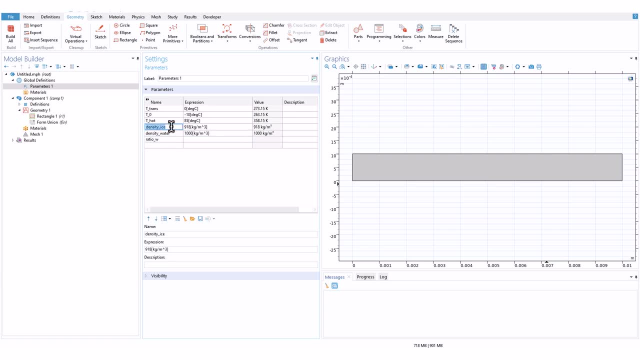 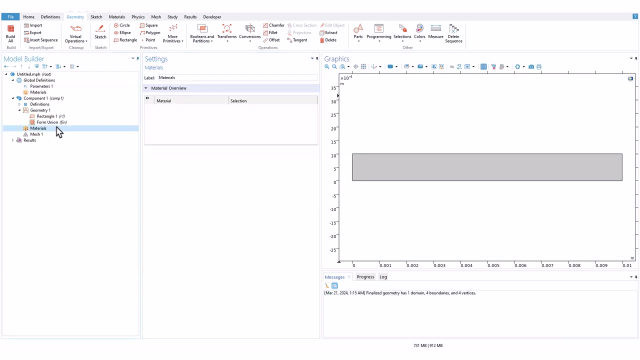 so that is the ratio of the ice and water. so i'll just copy and i'll divide and click on paste. okay, so this is the ratio of densities. so we are done with the basic parameter. now what we will do: we will add the material and then 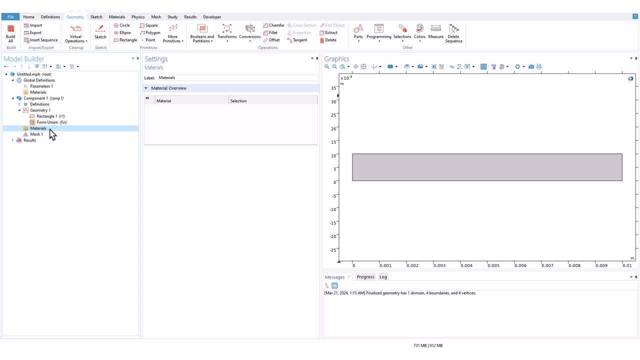 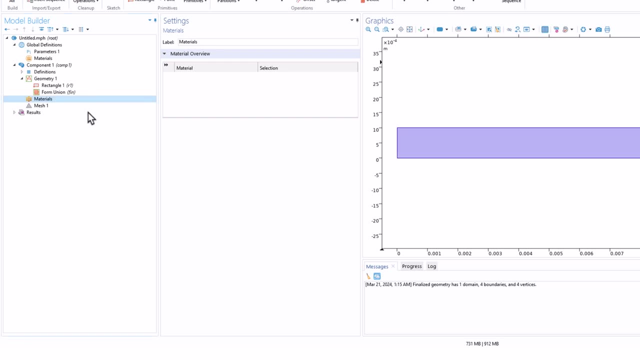 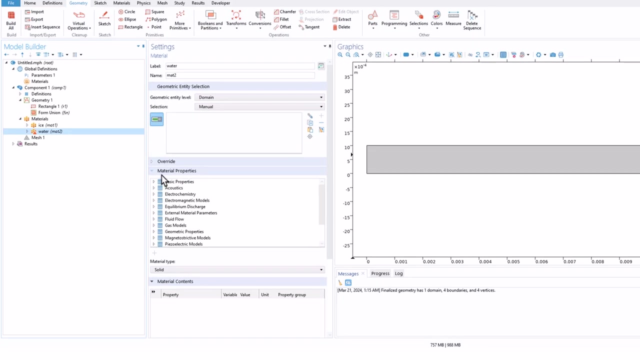 we can add the module in the physics, add the mesh and then model, okay, so we'll add a blank material, so this will be ice, and we'll again add a blank material. this time this will be a water. okay, don't worry, we'll fill in the details later, but for now i'll just select this. 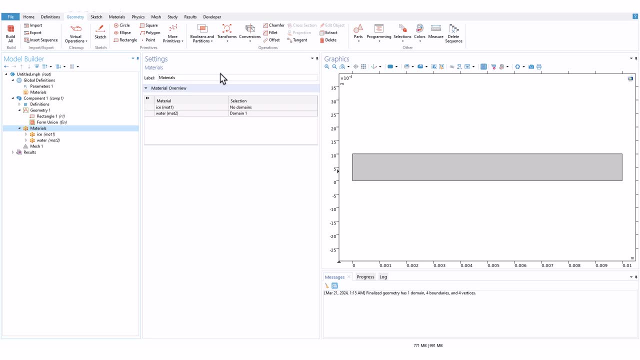 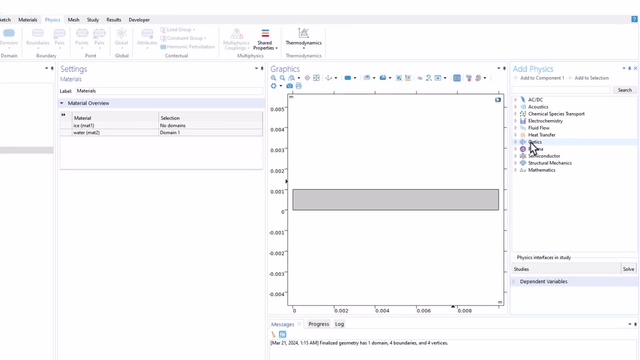 and what we will do now is that we will add the physics interface, so we'll go on to physics. click on add physics in the add physics, we'll. we are interested to study the heat, so we'll go to heat transfer and heat transfer in fluids because we will be studying water, so i'll click on add to component 1. 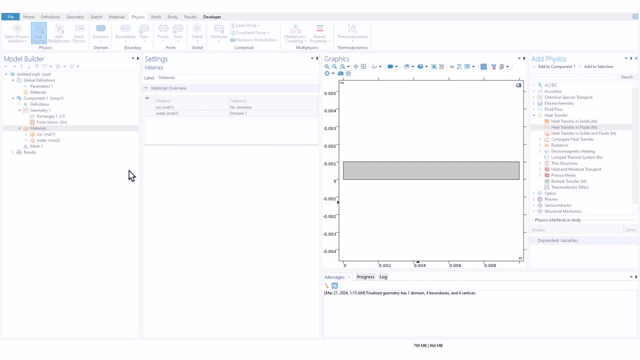 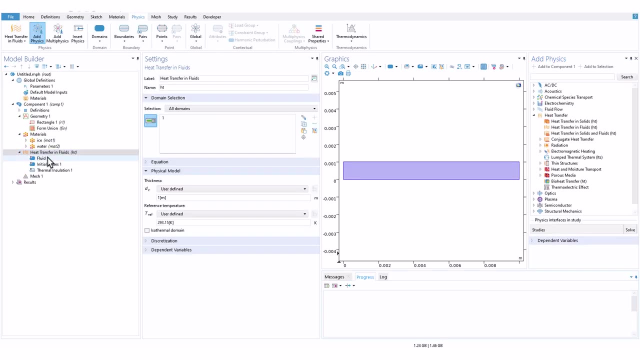 it might take few seconds, but that component will be added here just before the mesh, so you can wait few seconds. so the heat transfer in fluid is added. so i can close the physics because i don't need it now and, as you can see, the physics has already selected the block. now i'll go back to water. 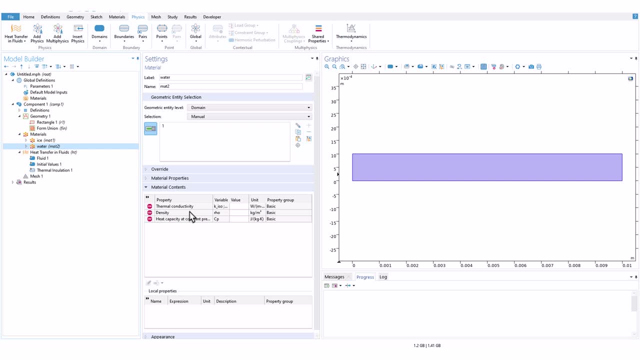 and you can see that it is asking for these three properties, that is, thermal conductivity, the density and the heat capacity. so let us write the values one by one. so what is the thermal conductivity? the thermal conductivity is 0.613. that i got somewhere from the tutorial. what by? 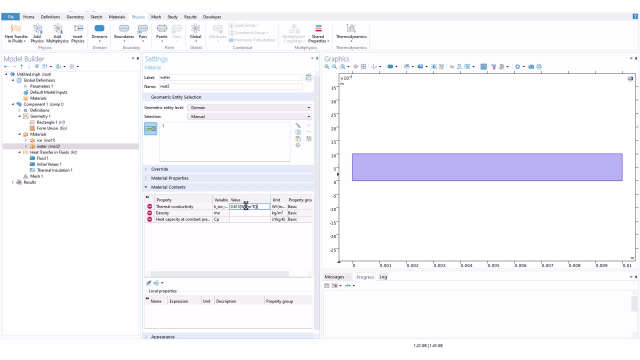 m into k times the ratio. uh, i'll just copy this. so i'll copy and i will just paste it. what is the error? i'm getting unknown variable ratio. oh, i think this is fine. now probably, yeah. so heat capacity at constant pressure. what is the value of cp of water? so the heat capacity of water is 4179 in si unit. 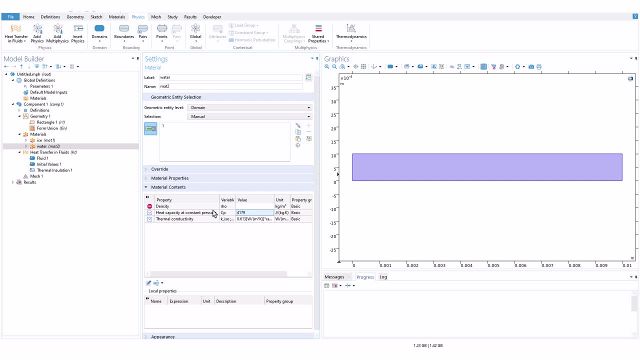 okay, and density. so the density of water is the density of water times the density ratio. why am i not writing only density of water? because remember that there will be a phase change and the density of water will not be fixed if we consider the total volume, the total density. 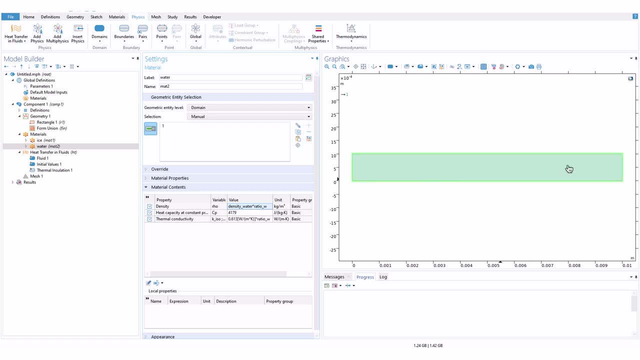 will not remain fixed. it will change with time, because the percentage of water will increase and the percentage of ice will decrease, and so on. so we are done with the water, and now we are interested to um write the properties of ice as well. so i'll just disable the water for now. now, 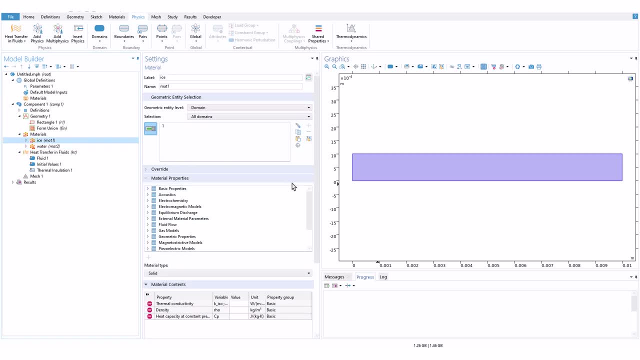 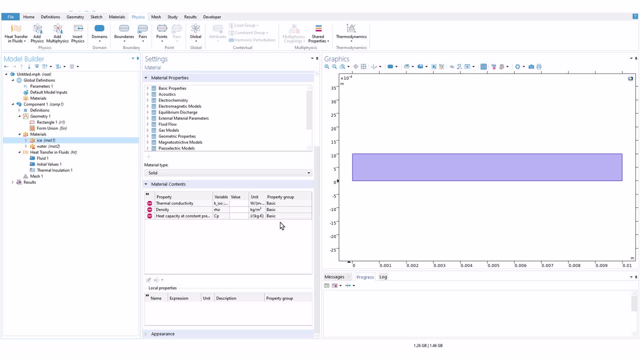 i'll just move this. so, as you can see, for ice also we need the thermal conductivity density as well as the heat capacity. so the heat capacity of ice is two zero um five two. so two zero five two. the density is density ice and the thermal conductivity. so thermal conductivity is around 2.3. so here we are writing. 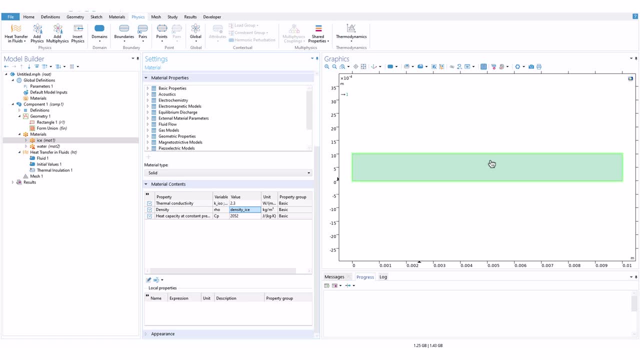 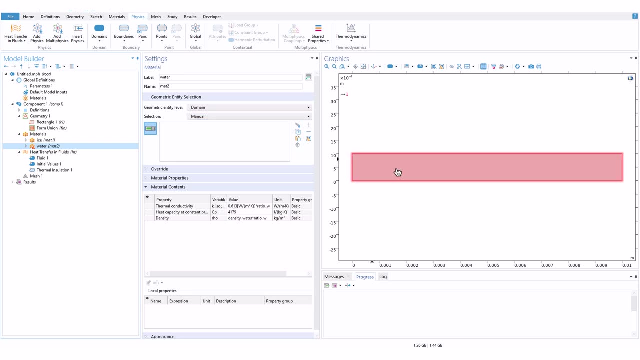 the density of ice, because initially the density of ice is the density of the whole block. okay, so we are actually done. now what we have to do is we need to set up the physics. so click on the heat transfer for fluid in the fluid, one section, right click and click on. 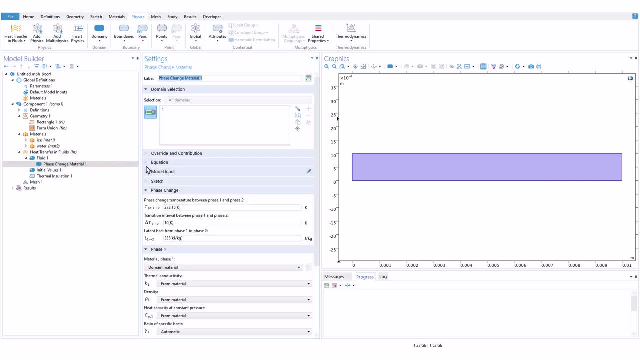 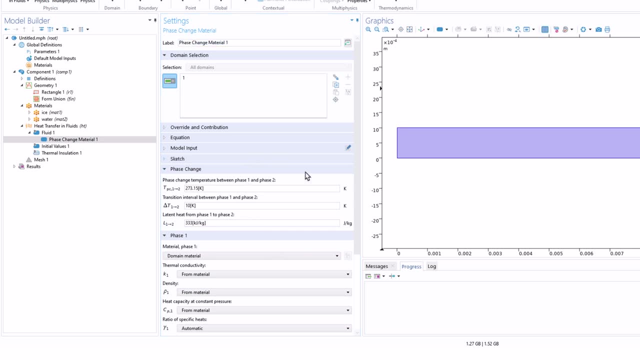 phase change material. when you click on phase change material, a lot of different settings will pop up and we need to actually fill in the values. so the phase change between phase 1 and phase 2 are: the temperature is at zero degree celsius. so this is fine, because the phase change between 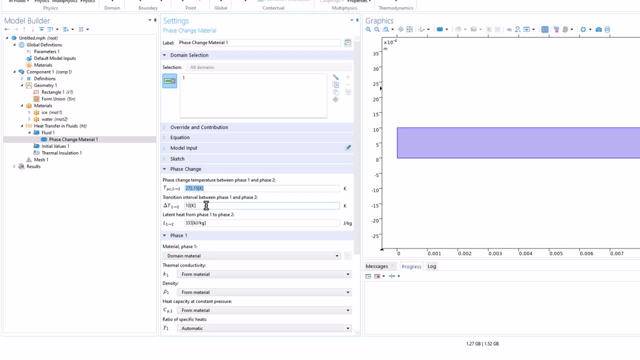 ice and water is at zero degrees celsius, so we don't have to change this. now, the transition interval between phase 1 and phase 2. what is the value of delta t? so for simplicity, let us take this as 1, 1 kelvin, okay, and the latent heat from phase 1 to 2. that means the latent heat of fusion. 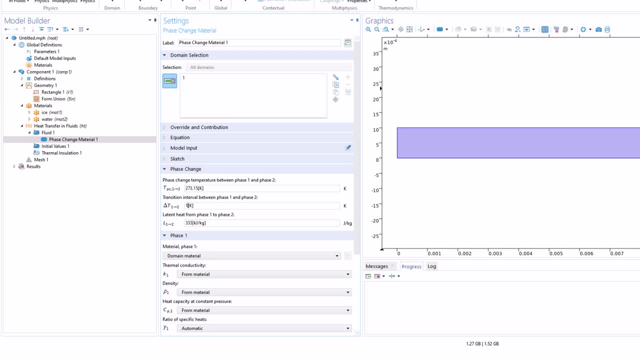 so we need to write the latent heat of fusion. so we need to write the latent heat of fusion. so i think it is 333. it's probably 333 if i am not wrong. so i i won't change this now. in the phase one we have to select as ice. remember that the phase change is from ice to water and not the 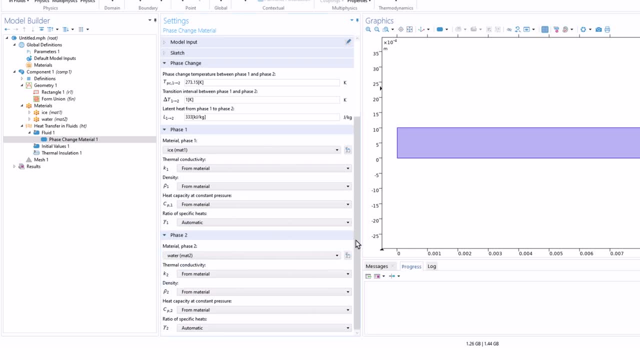 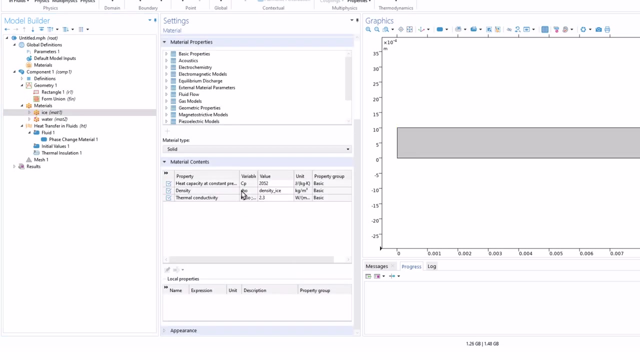 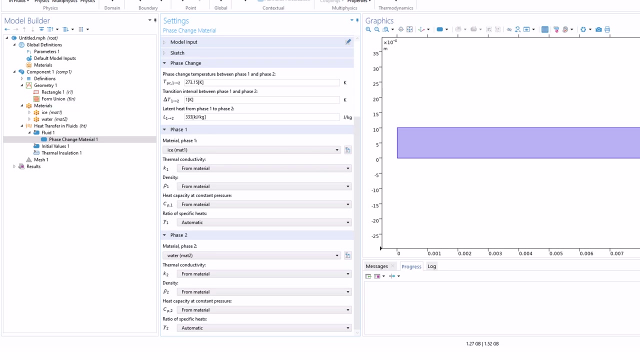 other way around. and the second is water and the rest of the parameter values we it will automatically take from the material component. so you can see that the density and other details are here already. that will automatically be taken from the material. so we have almost set up the 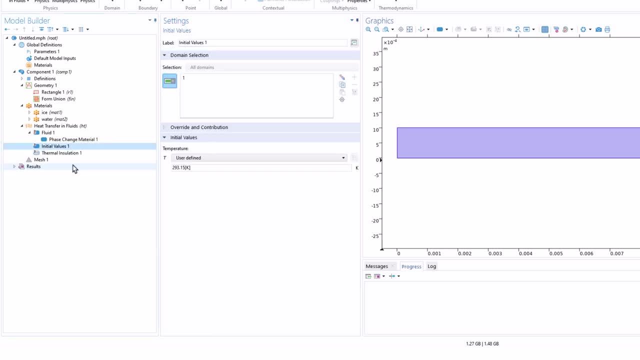 phase change. now let us click on the initial value. so what is the initial value of the temperature? is it is really Celsius? no, we have to select the initial value of the temperature. so we have to set up- already set up- the initial value. so that is t underscore zero. remember that this was our. 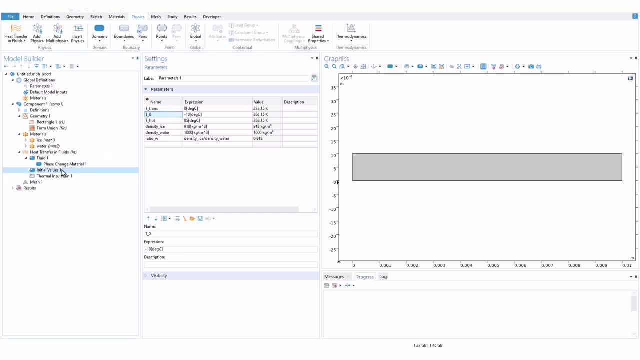 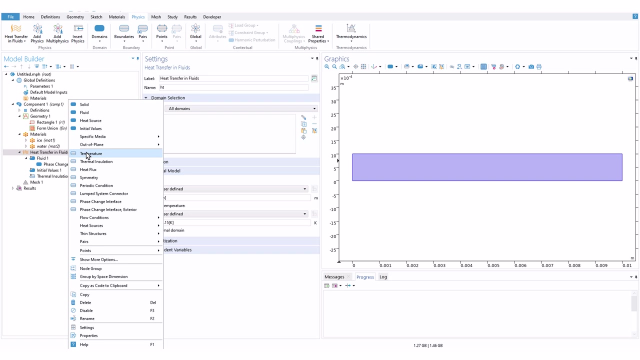 initial temperature. that is the value of temperature of ice. now we need to add the thermal insulator. by default, you will see that the insulator will be added, so we don't have to worry about that. and we have to add the temperature. so I'll click on temperature. 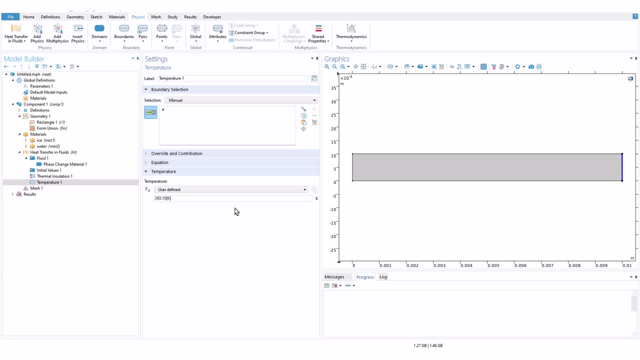 so here's the the interesting part. we will create a step function and the temperature profile will be in the form of the step. so what we'll do? we'll go on to global definition in the function. we'll click on step and here we'll write t input and here we will write t. 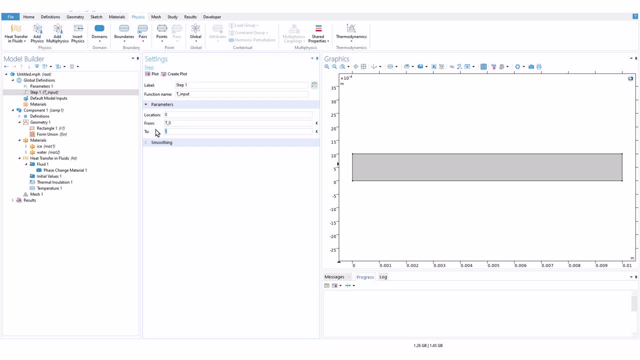 underscore zero two. I'll just copy this because, uh, I generally don't remember the value names, so let us see how the plot actually looks. it looks something like this, so I think this is fine, but we can, of course, uh set the location, so we can set it to 0.04. 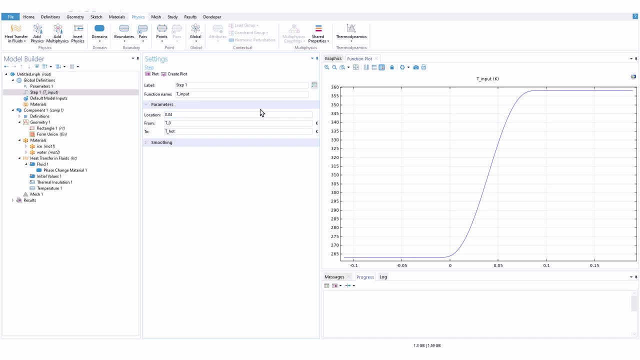 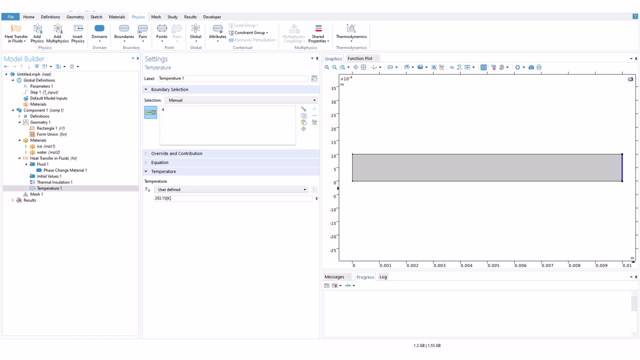 yeah, this is fine. so we have set up the temperature ramp, okay. so here what we can do: we can call the function t input and we can actually the setup the temperature. so we will just paste and within brackets we can write t. that is the time a by default in fossile multiphysics and. 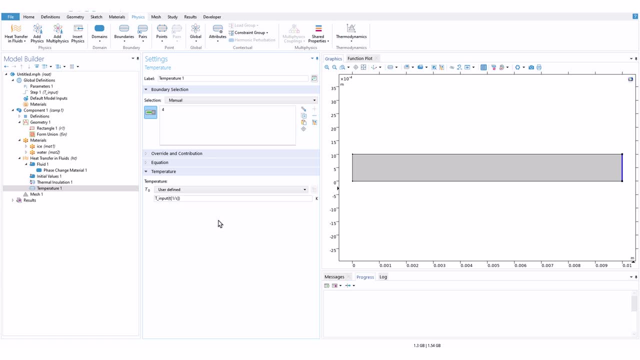 to state consistent with the unit, we will write 1 by s, okay, so this is the format you generally use to write the time Dependence and also to keep consistency with the unit. so we are almost done. now let us create the mesh. to create the mesh, what we need to do, we just click on first, build all and see if it is working. 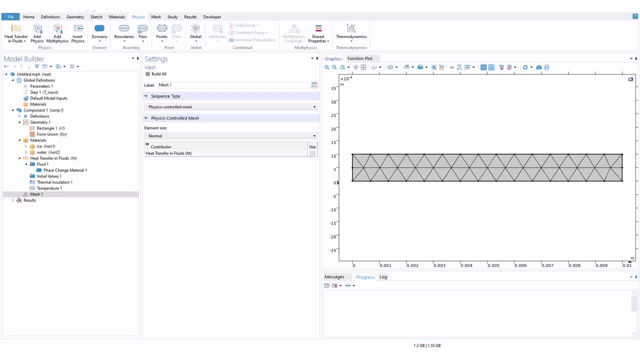 fine, but i am not actually happy with the default mesh, so i'll just go on to mesh, click on distribution. but yeah, i'll just click on user control and i'll just click on distribution. i'll select these two sides. maybe i will add 50 elements. 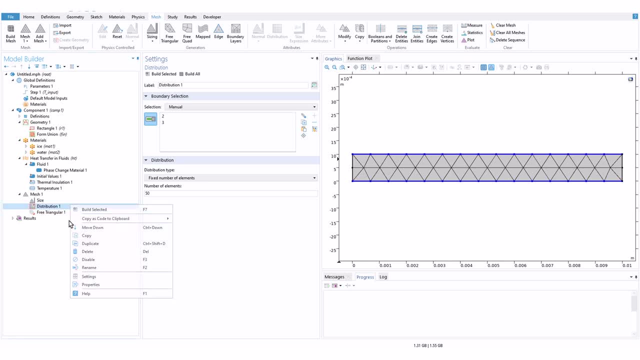 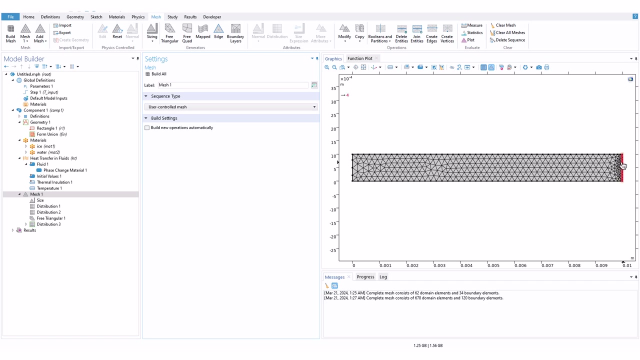 and i will just duplicate this distribution. click the and maybe i'll just add 16 elements here. then free triangular, i'll keep the remaining and maybe i can add a distribution here. let's see. yeah, so the mesh is almost done, so i try to add a final measure because there will be a temperature. 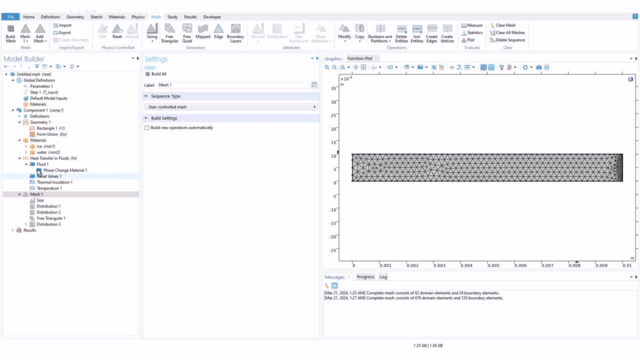 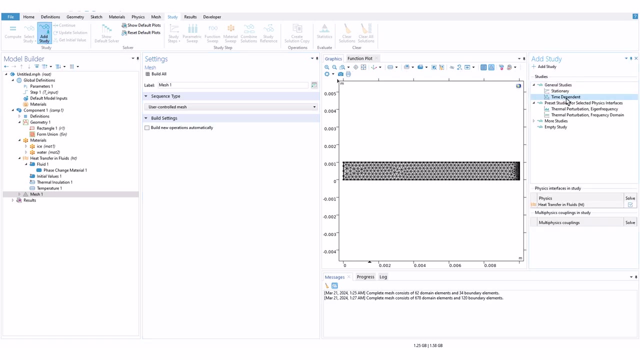 gradient towards the end. so we are almost done. now the next part is to set up the study. so we'll go on to study, click on add study, and we are interested in a time dependent study. so just right, click, click on add study. again, it might take few seconds. if your system is a bit slow, don't worry, so in the time 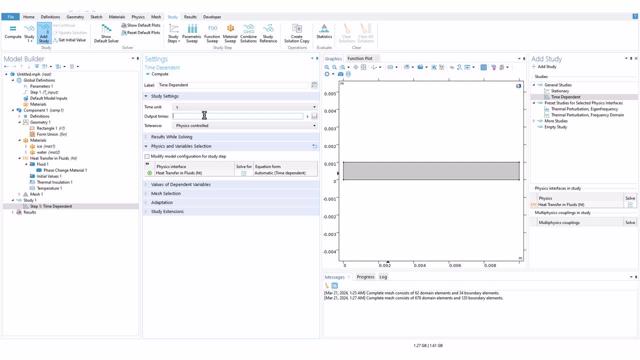 there will be nothing in one second. so if you think physically, let's say you have a ice cube- how long does it take to melt? um, it generally melts in 30 seconds to maybe one hour or few minutes. so we'll first set the range from zero to 20. 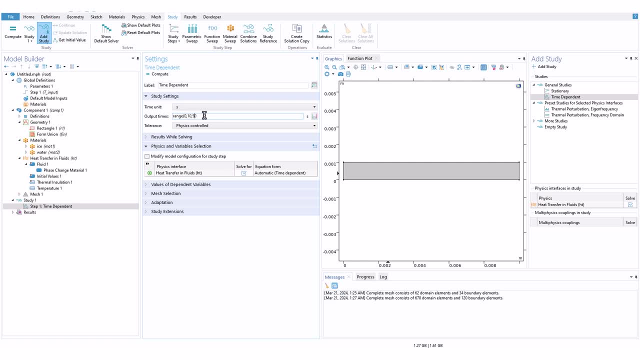 or 0 to 10 to 50.. and then we'll set a range from 60 to 20 to um 120.. and then another one that we'll set is the 4x125 range from c formal range up to 20 range llev산, or 0 to 510 or 0620 range enc Dunkity college range deck for 15 months not covering 29 formula range, 10, formula range 30 into sc 600 data super synagogue practice 20SP, cognitive Kunihama series centeremos그램 will set again the math within an arm. 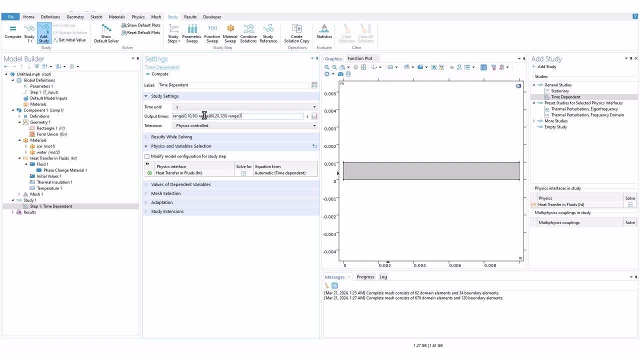 then another range from 120 to 60 to 1100. okay, and I'll just change this to 100 to keep it consistent. so I think the values are not overlapping. I hope this is fine. so maybe I can change this to 1300 or a multiple of 60, so 1200 is fine. 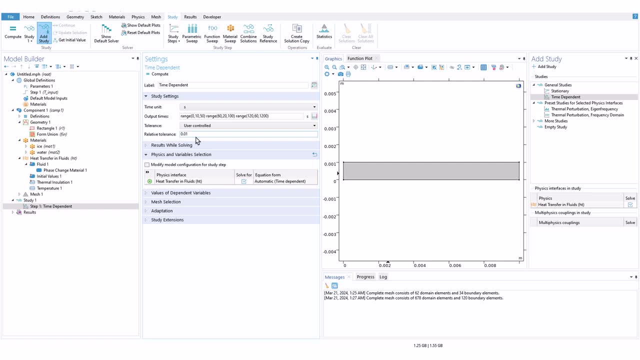 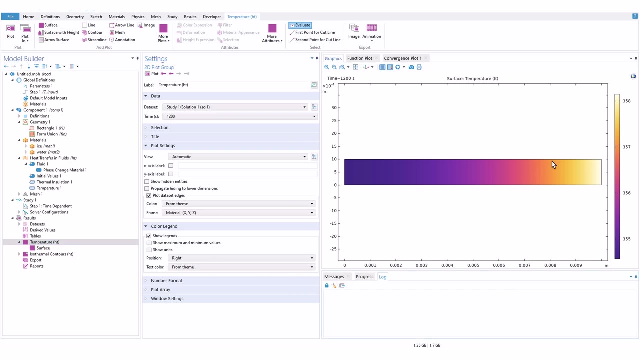 I guess let's see, and in tolerance we'll just set it to 0.01 and we'll click on compute. so let's wait for the result. so the simulation is done and you can see that the temperature gradient is shown here. now I'll go on to 10 seconds. I'll 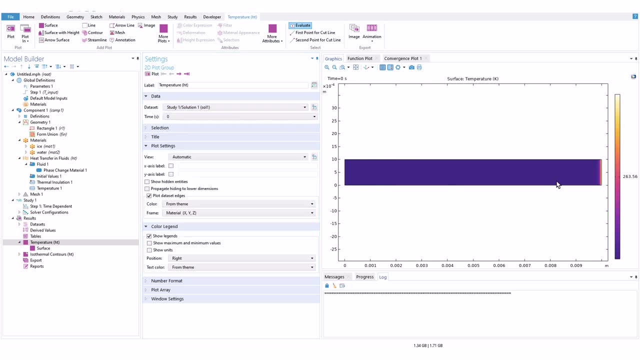 first go on to 0 and click on plot so you can see. initially it is all ice, so 263 Kelvin is basically minus 10 degree Celsius. so I'll go on to surface and instead of Kelvin I can just select degree C. click on plot. now you can see. 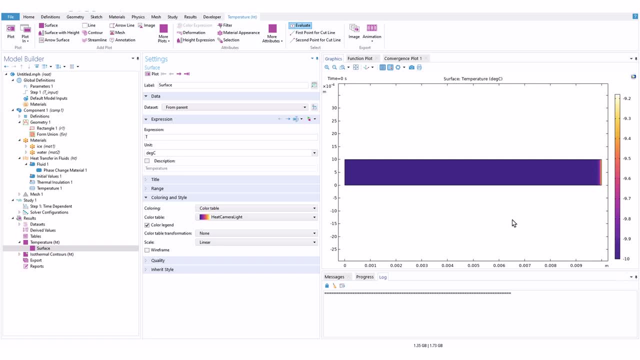 that the plot is in Celsius, so it is minus 10. now, if I go on to higher temperature, let's say 10 seconds, you can see that the temperature is actually rising. so this end is around 85 degree Celsius, as we have set it to 85 right, and the colder region is around minus 10, and 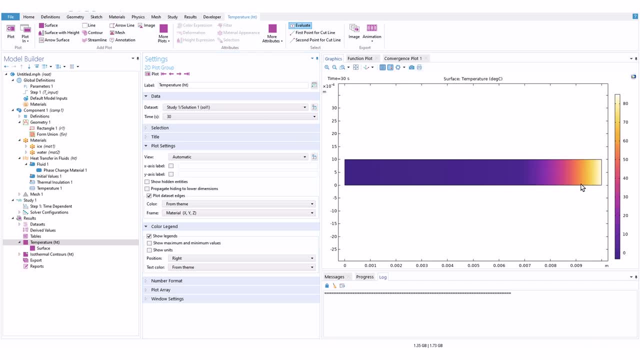 after each time you see that the temperature is actually increasing and basically the ice is melting. so if I click on 420, you can see that all the ice has melted. why? because the temperature gradient you can see is close to 30. that means it has already melted into water. so if I click on 360, 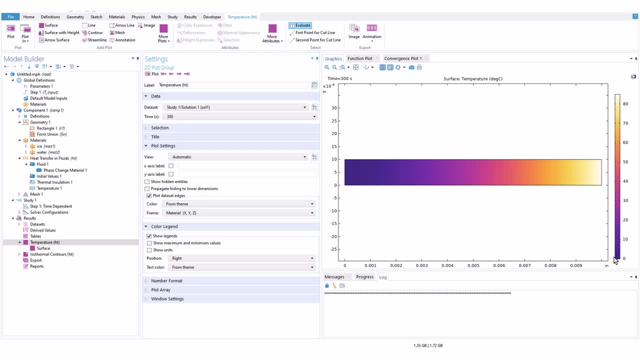 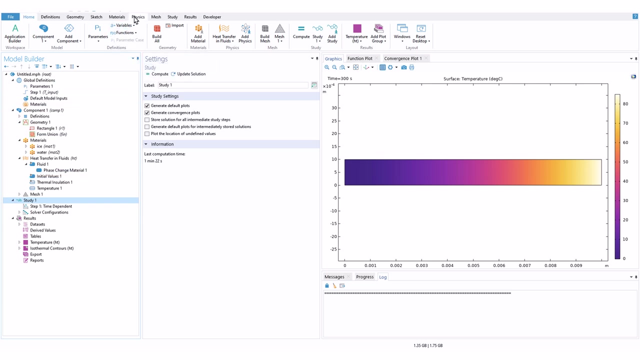 it has melted 300, so probably after 300 second, all the ice has melted. oh, it is all gone, so I can just something like that, okay, so this is the new okay part that I wanted to show you. I've saved it as from theób считable. 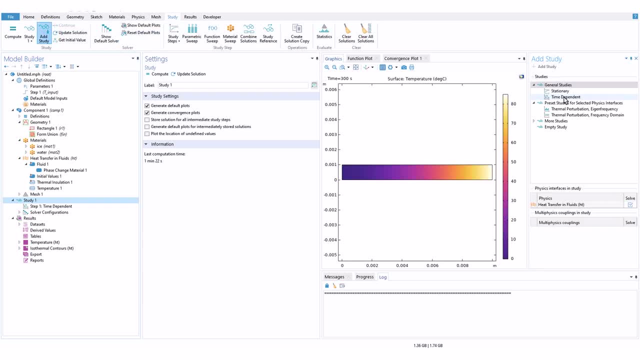 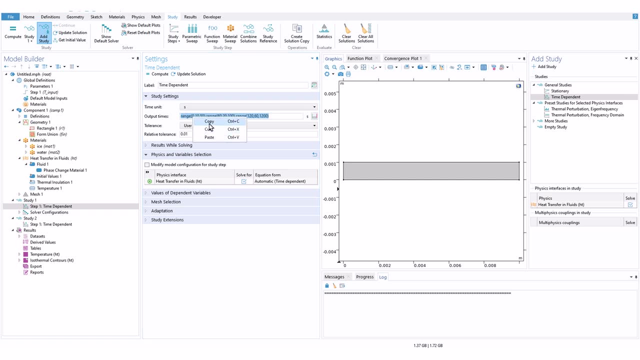 sequencer. so if I was going to tell you guys to duplice the peak of max film there, probably I'll be coming up with something like this, something like that. okay, so now what we can do, we can actually add another study and then simulate it to get the result without the latent heat, and then we'll compare the results. so I'm going to add study. we again add a time: dependent is steady. to save time, I will just copy the range pasted, the main orange, go to program and try to scale, will use a setting又. 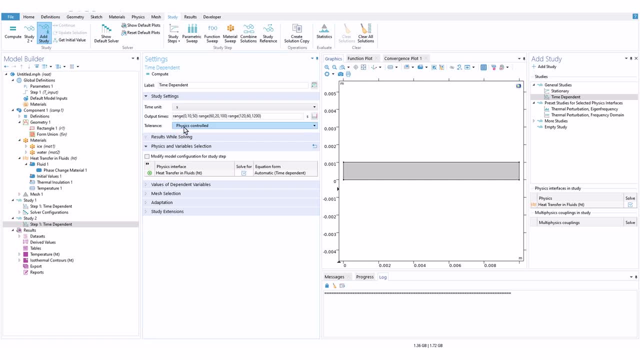 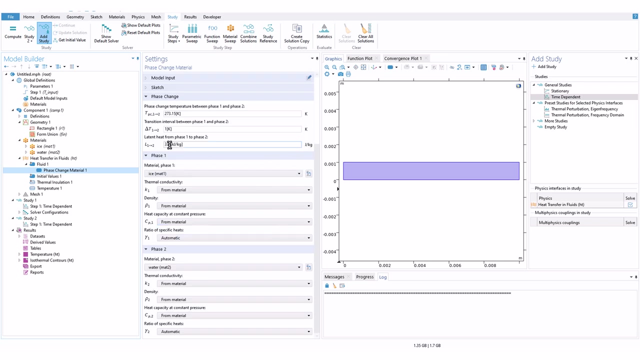 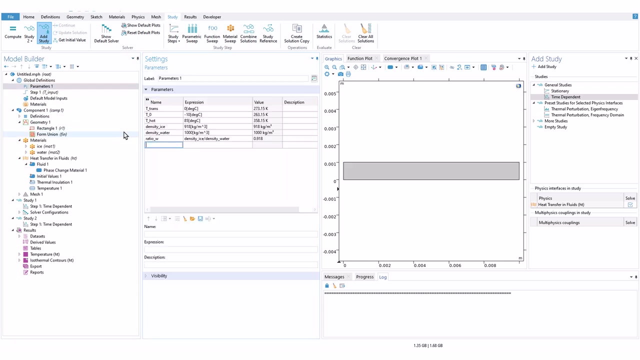 or the nósuda and پ呵 wellness is possible, available here, and I will just add the sweep, add the latent heat. so I haven't set the latent heat here. what I can do is and go on to the physics. and here what I can do I can just cut latent ice, okay, and here I will create and I'll paste the value. 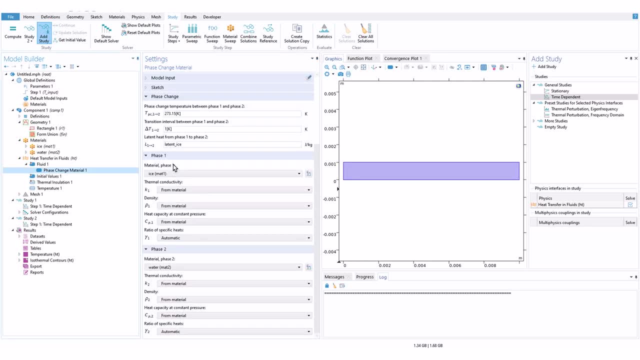 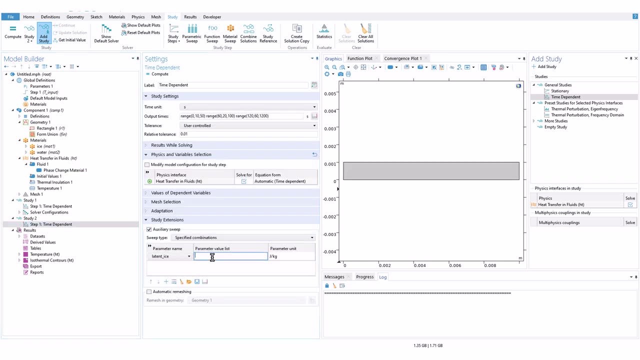 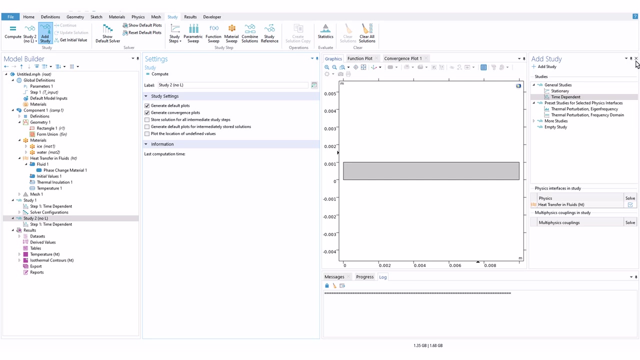 okay, now I think this is fine. yeah, so I will go back here and I will choose the latent ice and set it to zero. so basically I am NOT considering any latent heat of fusion in this case, in study 2. so here I will just write: no L, okay, and now I will click on compute and see the results. so I'll just 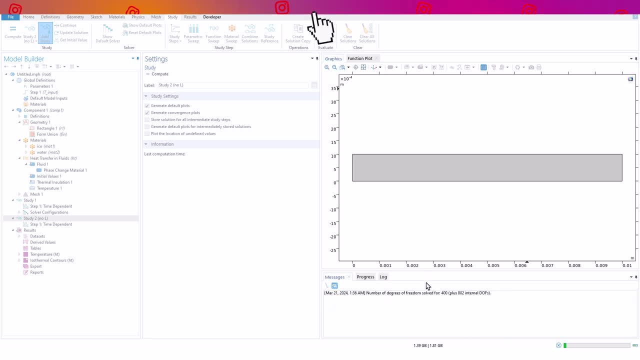 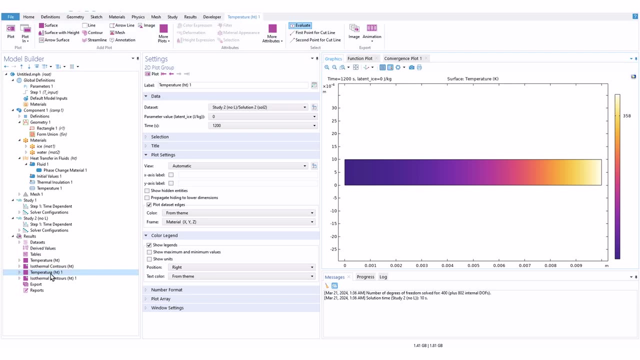 wait for the results. probably this will take less time because because it will now not have the latent heat calculation. so this is the latent heat calculation. so this is the temperature profile now in the two. this is the temperature profile now in the two-dimensional plot. you won't see much. 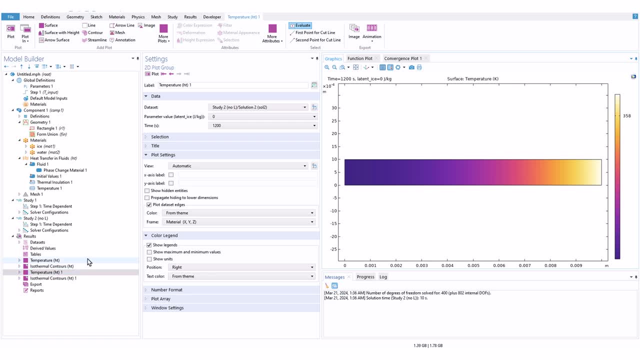 응 of a difference. the difference will be prominent when we will plot the one-dimensional graph. so I'll go on to result: click on 1d plot group and then we'll click on line graph. I will click on driven path and I'll highlight here line time length, because the data is not calculated just to see the value of the Δ Hard Dashing. 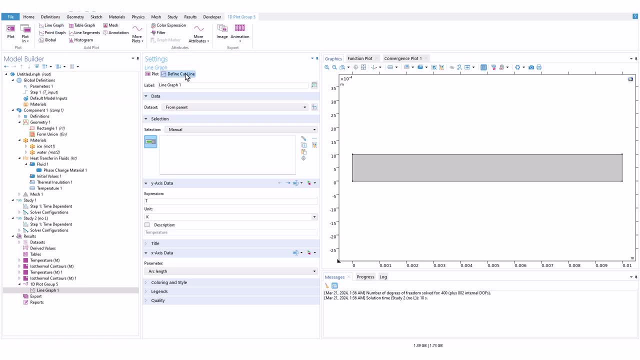 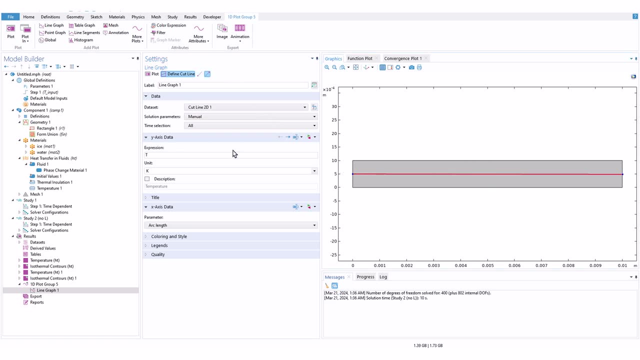 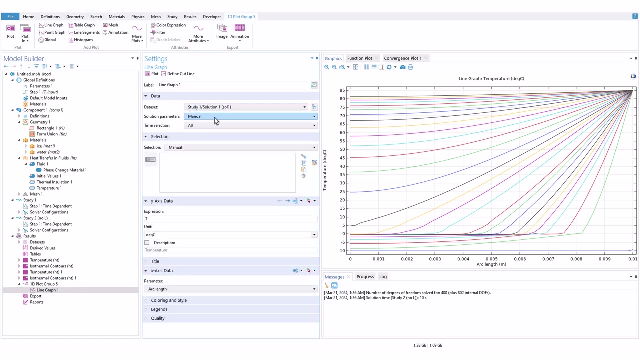 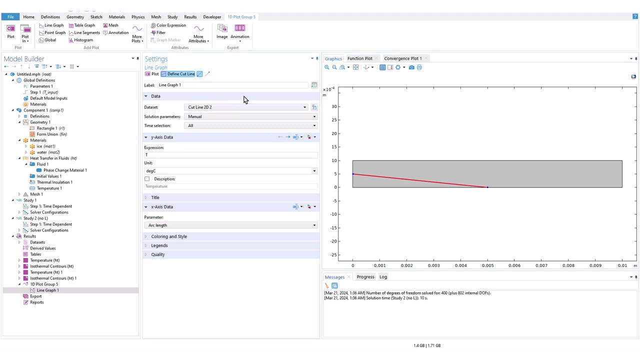 Now I'll click on define cut line and we will just set two points just to check the result and the temperature will select degree Celsius and click on plot So we can select solution one. define the cut line once again, So we can select this and click on plot. 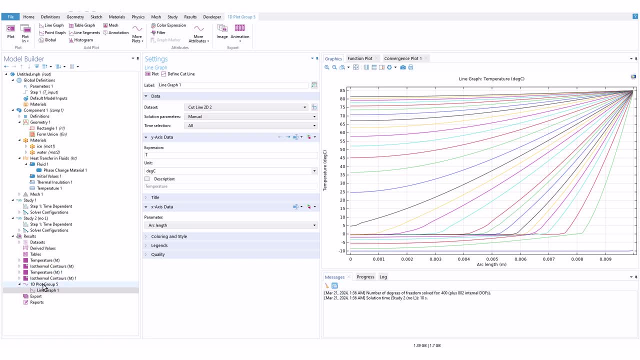 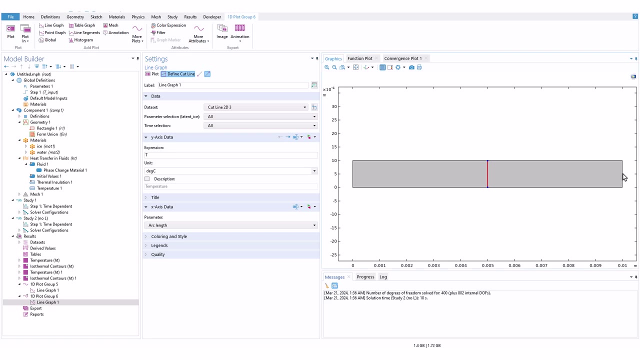 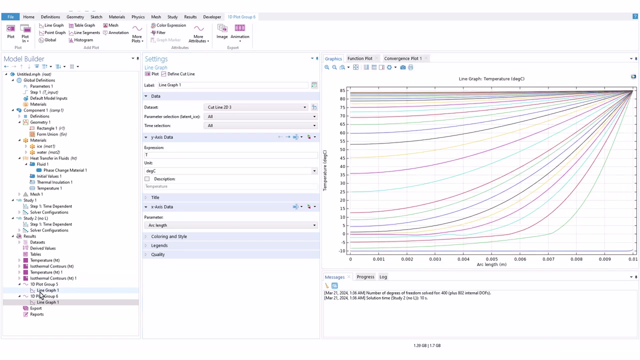 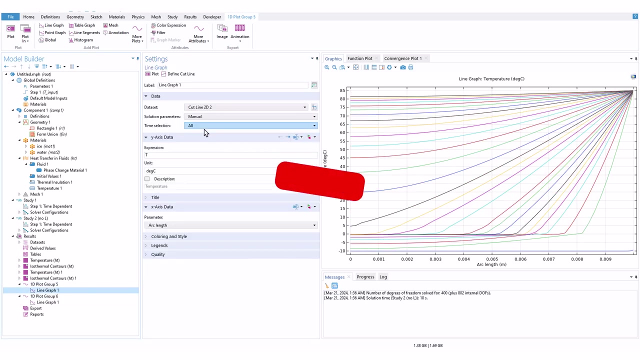 So this is with latent heat. So let me just plot this once again. I'll just duplicate this And this time I'll select the second solution And again I will choose the points and click on plot. So let us first see the graph with latent heat and try to understand what is going on. 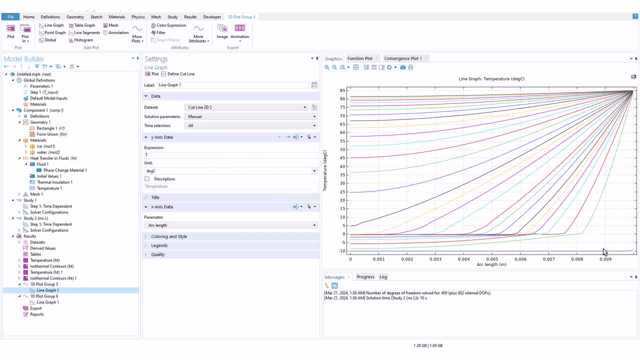 Now you can see that at lower time, that is, at zero second, all of them is at minus ten degrees Celsius. Now, at some higher time Some of the ice has melted and at zero degrees Celsius you can see it is getting flatter. 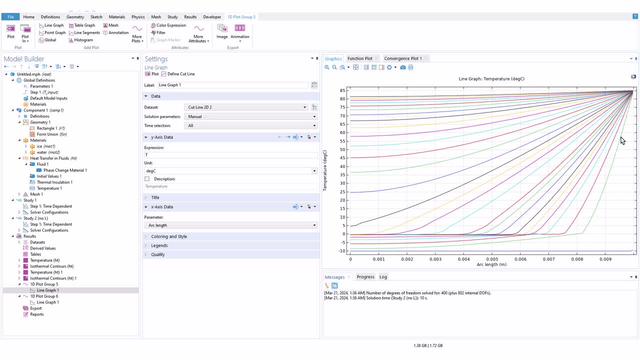 because of latent heat of fusion. So it is suddenly changing. The curve is having a sharp pointy edge. here You can see why: Because the water and ice interface, the temperature is actually zero degrees Celsius, because ice is melting into water Without actually increasing the temperature. 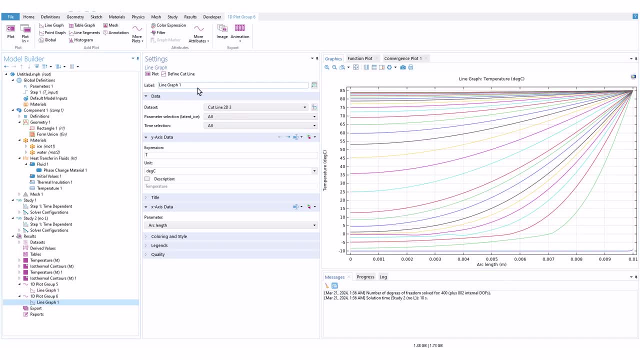 Now, if you look at this graph without the latent heat, you can see that the curve is actually smooth. Why? Because here, in this case, the latent heat of fusion is not there. It is zero. That means it has nothing to resist the change in temperature. 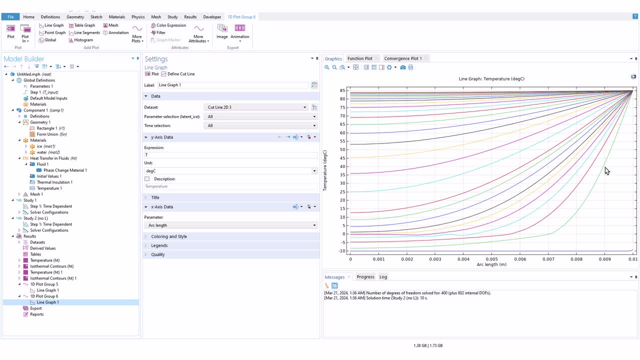 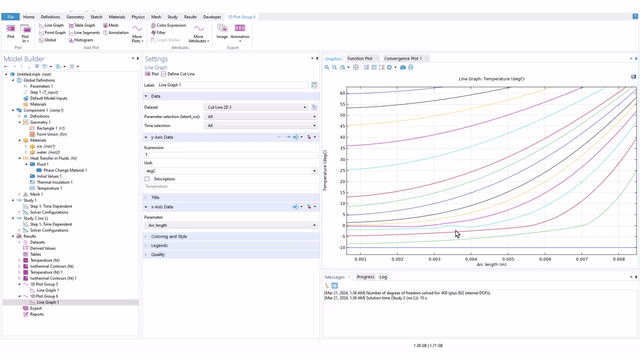 So the ice will easily get converted into water. So at higher temperature It will gradually melt. So It will gradually convert it into lower temperature without any sharp change, at zero degrees Celsius. Don't worry about these discrepancies. It generally arise if the mesh is not finer, and so on. 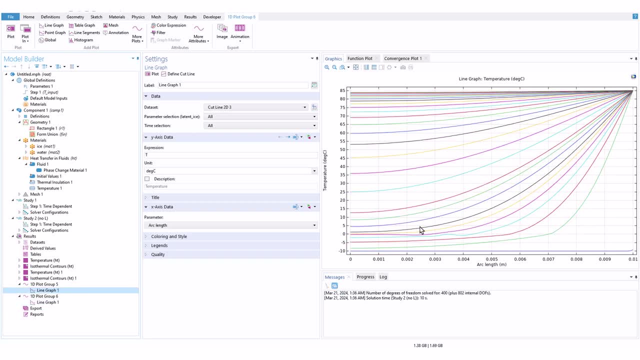 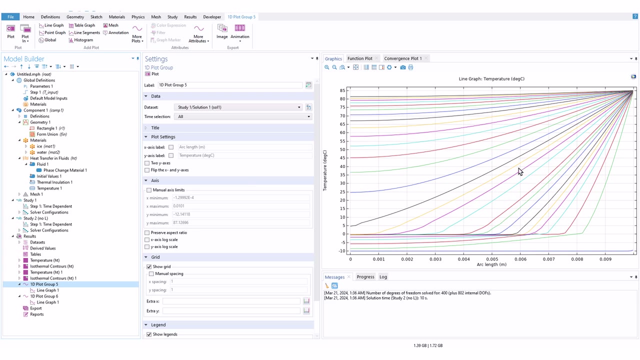 But if we just look at these two graphs, you can see that clearly there is a visual difference between the graph using latent heat and the graph without using the latent heat. So this is the main inference of this work. And of course You can do various other studies, other plots, two dimensional plot, time dependent plot.